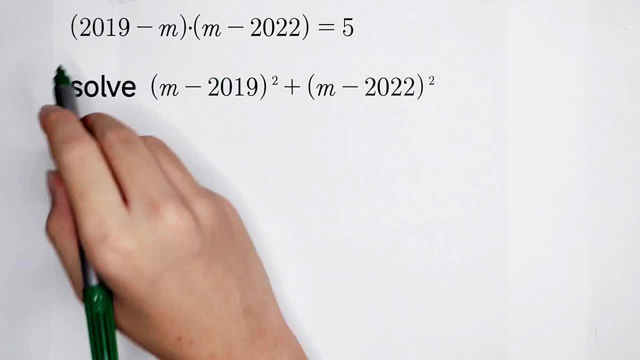 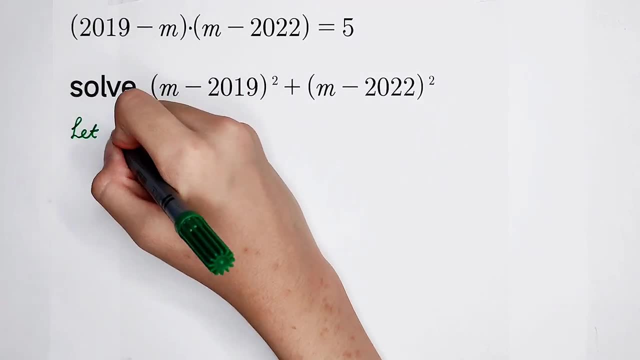 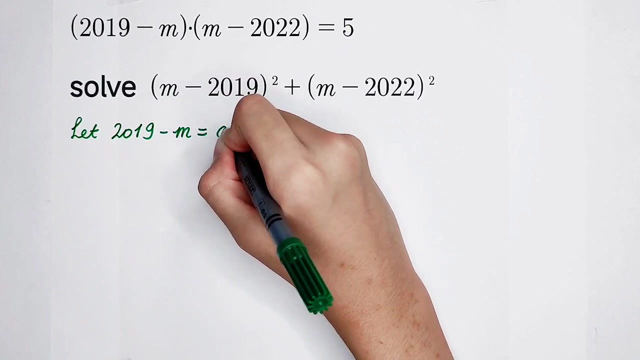 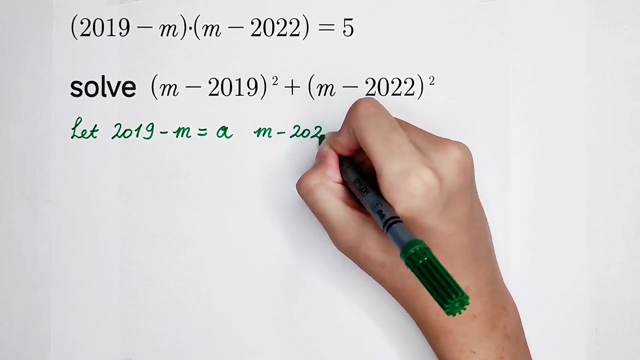 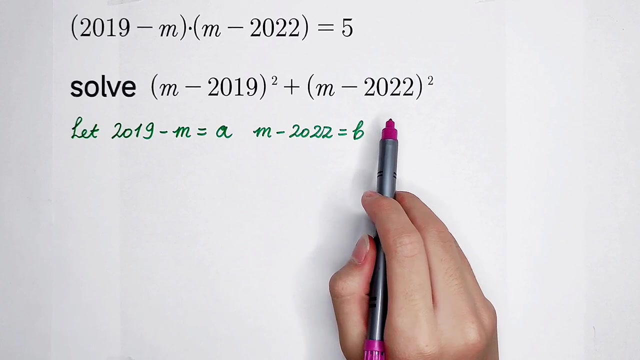 Then we have to let them. For example, I let, Now I would like to let: 2019 minus m: It is a, And m minus 2022, it is b. And then this: it has to be written into the term of a and b. 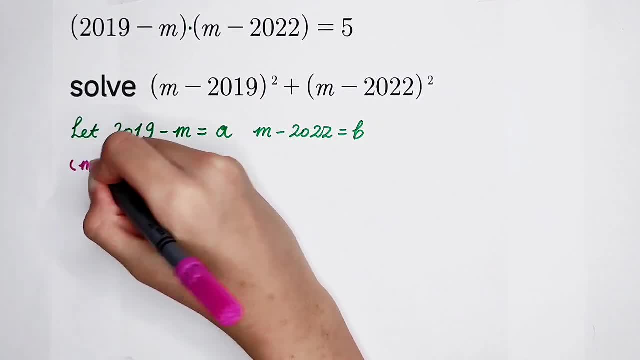 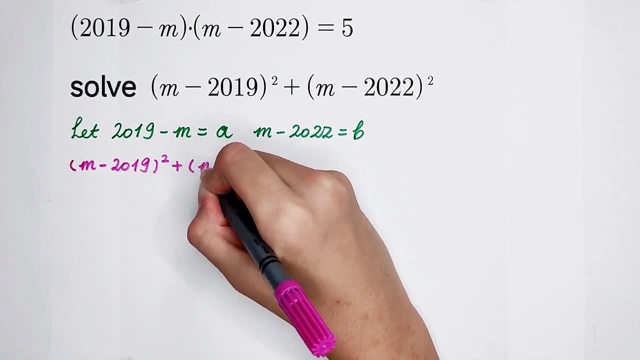 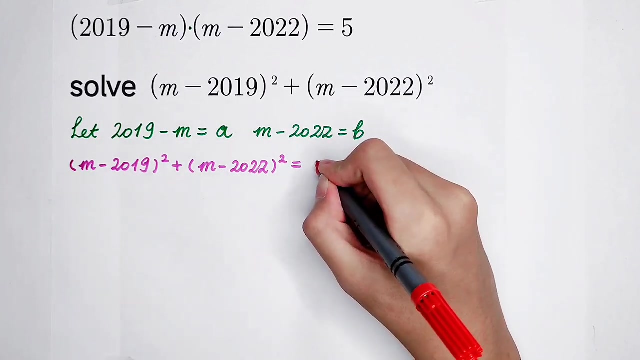 Now I write it here: m minus 2019, all squared. and then plus m minus 2022.. All squared, Okay, Because 2019 minus m, it is a. So m minus 2019, it is minus a. 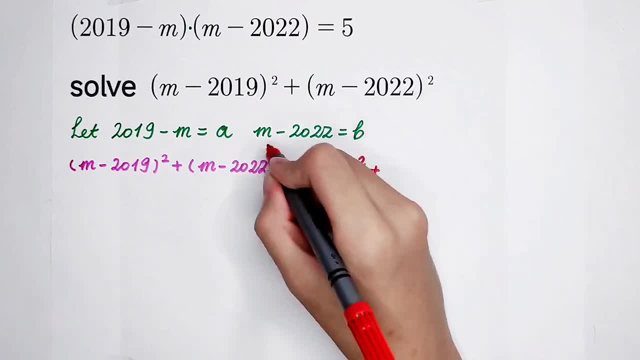 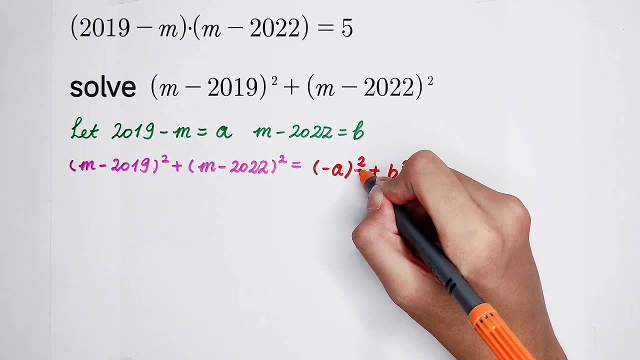 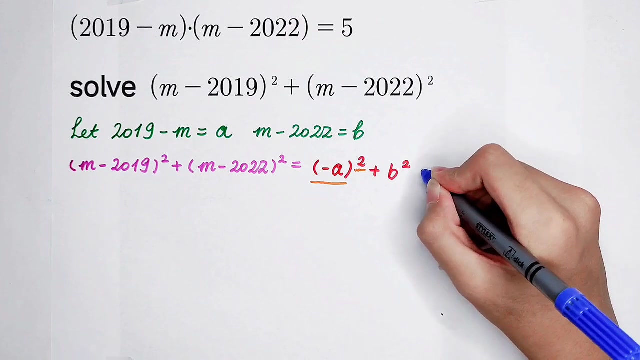 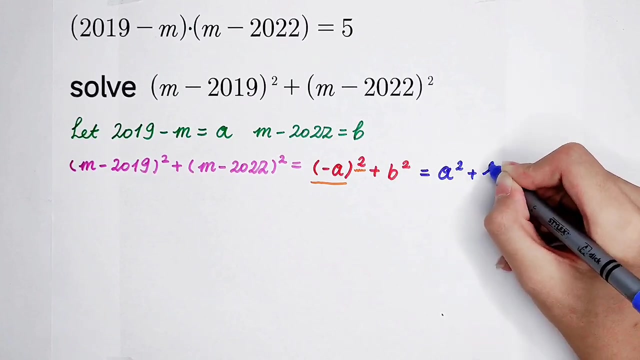 Then all squared, Plus this is b Squared. And now, because here it appears as squared and the base is minus a, Minus a, then squared, it is equal to a squared. So because of this it is just. it is just equal to a squared. then plus b squared. 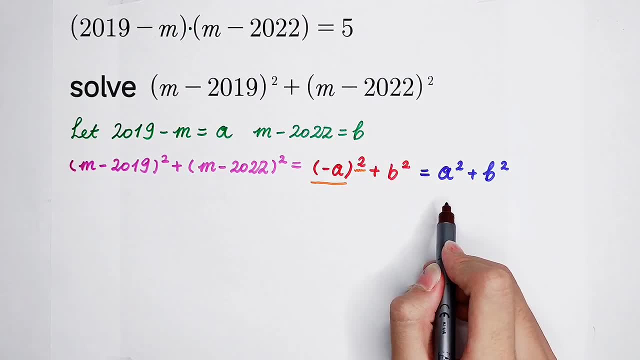 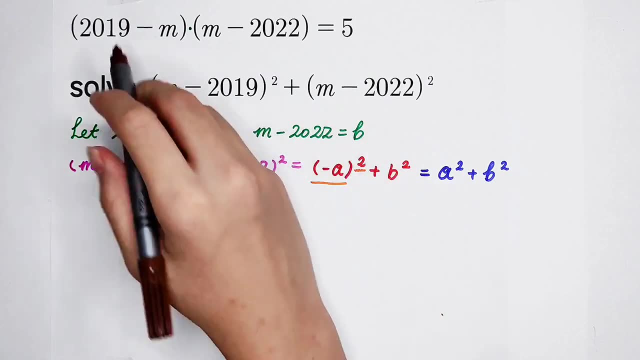 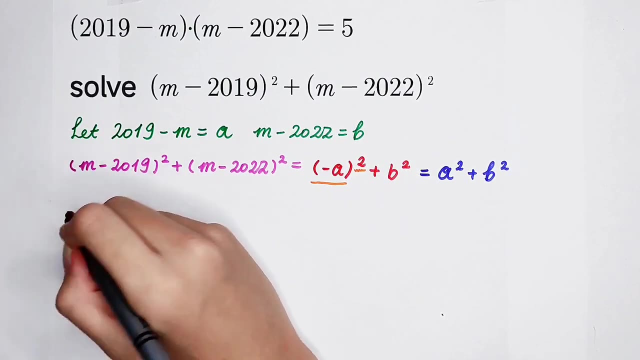 We just solve a squared, then plus b squared. It is okay. I have to get an equation set of a and b, Because this times this, Yes, it is equal to five. So the first equation I can get that is a, then times b, it is five, isn't it? 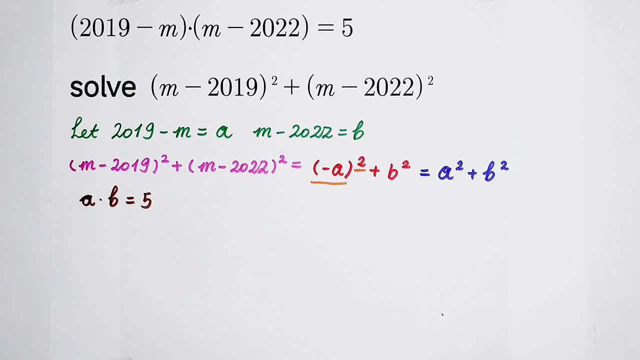 And the second equation is: we pay attention, here a. here appears an m, but the coefficient of it is negative one. But here The coefficient of the m it is one Minus one, and here positive one, Negative one, positive one. 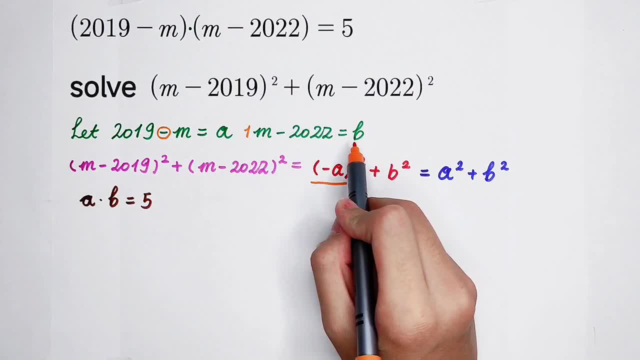 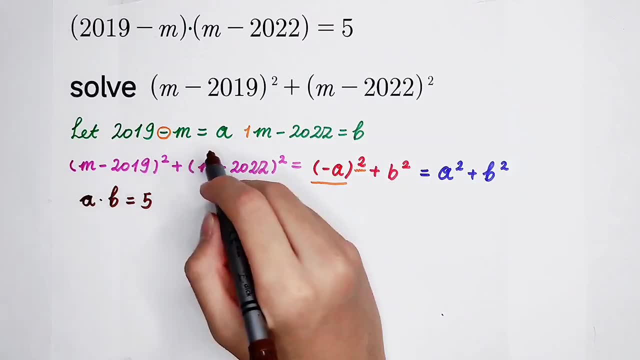 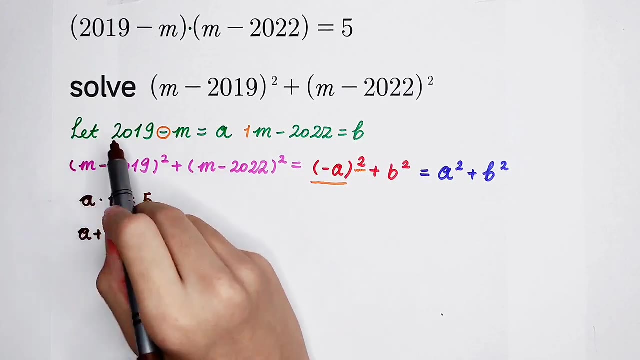 If I add a and b together, then minus m positive m cancel. So a plus b, It is 2019.. And then minus And then minus 2022.. Negative m positive m cancel. So they are canceled, and don't worry. 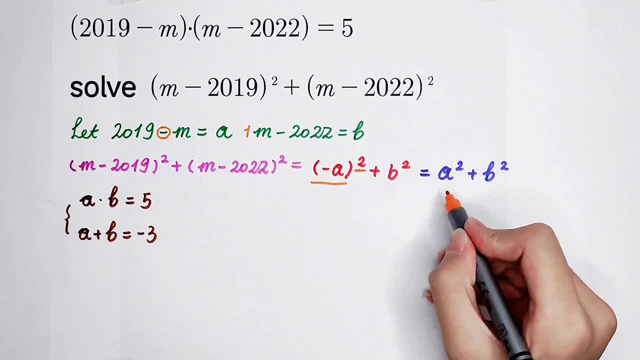 From here, our job is to find the value of a squared, then plus b squared, Just from the multiplication of them and the addition of them. I have to remember you, Have you remembered this formula, The first binomial formula: a plus b, all squared. 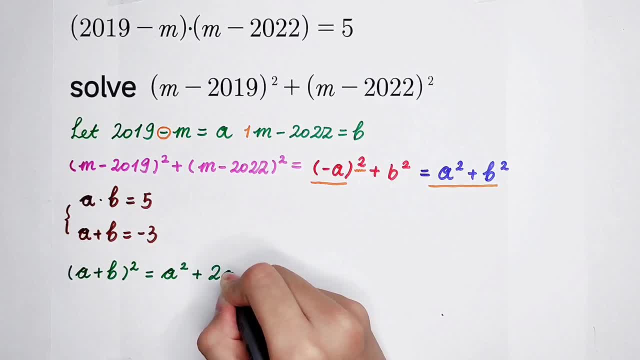 It is a squared and then plus two times of ab and then plus b squared. If I let, I just do some changes from this formula Now. I would like to let a squared, then plus b squared, be on the left-hand side. 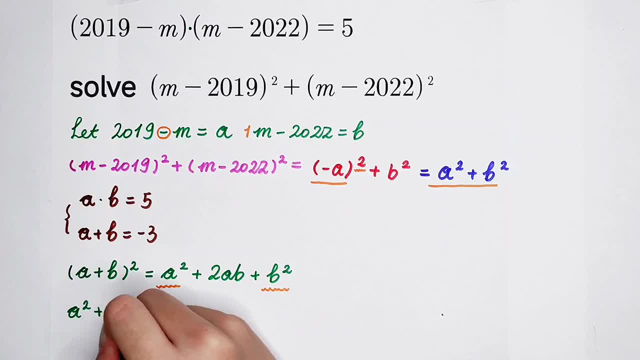 And I move. I just remove this from left-hand side and move it to the right-hand side. That is a plus b and then all squared minus two times of ab. Then I just from this because a plus b, we know the value of it from this problem. 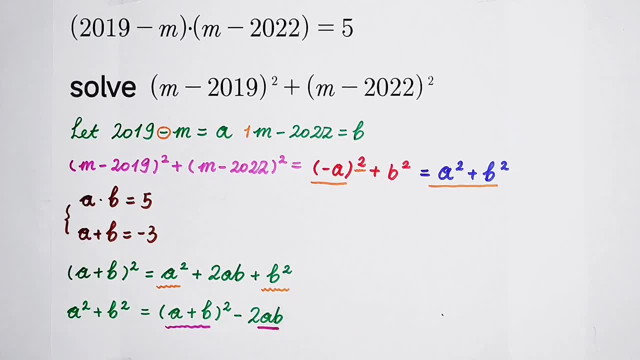 And it is a squared And a times b, the multiplication of them and the addition of them, Then a squared, then plus b squared. It is just a plus b is negative three and then squared minus two times a times b is five. 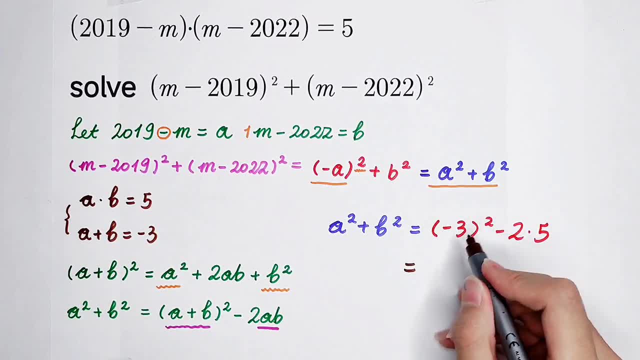 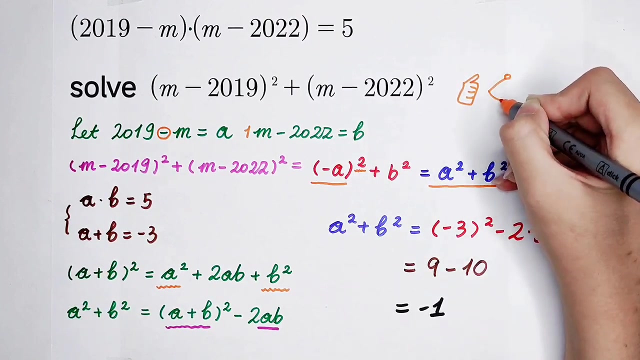 This negative three, then squared, it is three, squared, It is equal to three squared. Three squared is nine And then minus two times five is ten. So the final answer is negative one. Did you get it? And don't forget to give me thumbs up, ring the bell, subscribe me and we see you next time. Bye-bye.